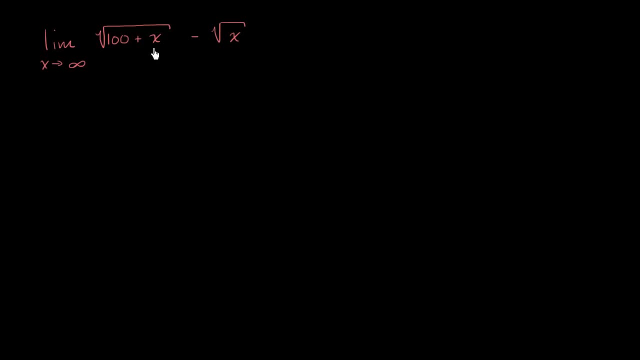 So first let's just try to think about it before we try to manipulate this algebraically in some way. So what happens as x gets really, really, really, really large, as x approaches infinity? Well, even though this 100 is a reasonably large number, as x gets really large, billion, trillion, trillion, trillions. 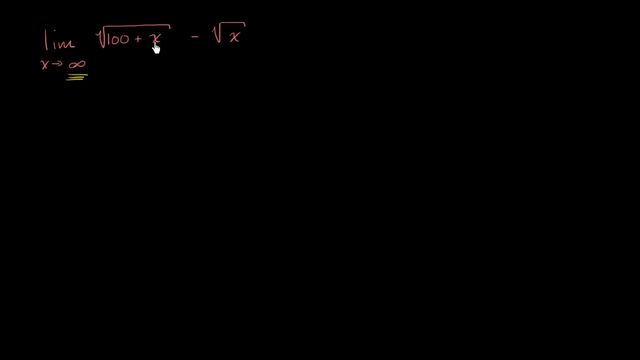 even larger than that: trillion, trillion, trillion, trillions. you can imagine that the 100 under the radical sign starts to matter a lot less As x approaches really, really large numbers. the square root of 100 plus x is going to be approximately the same thing as the square root of x. 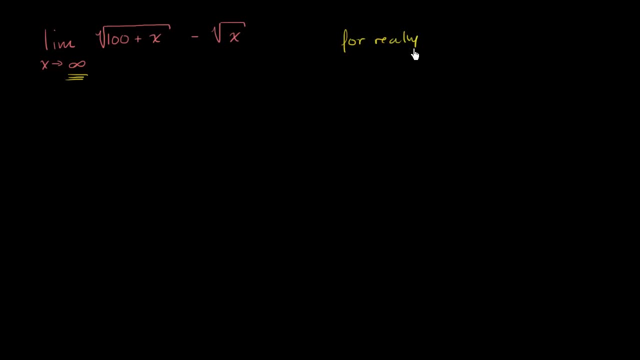 So for really really large numbers, large, large x's, we can reason that the square root of 100 plus x is going to be approximately equal to the square root of x, And so in that reality, and we are going to really, really, really large x's. 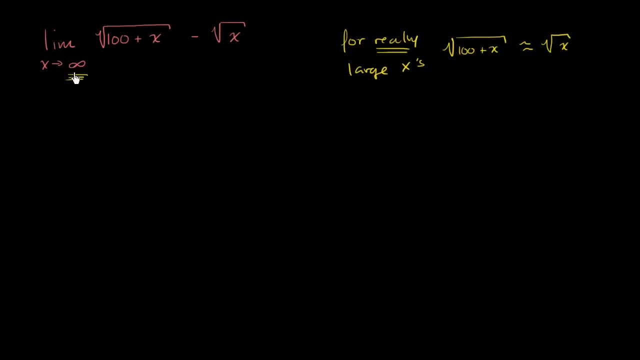 in fact, there's nothing larger where you can keep increasing x's that these two things are going to be roughly equal to each other, So it's reasonable to believe that the limit as x approaches infinity here is going to be zero. You're subtracting this from something that is pretty similar to that. 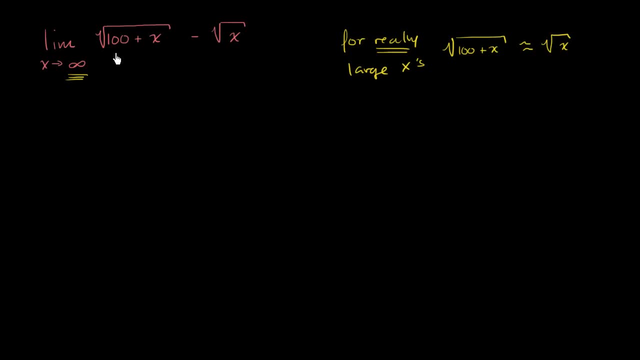 But let's actually do some algebraic manipulation to feel better about that, instead of this kind of hand-wavy argument about the 100 not mattering as much when x gets really, really, really large. And so let me rewrite this expression and see if we can manipulate it in interesting ways. 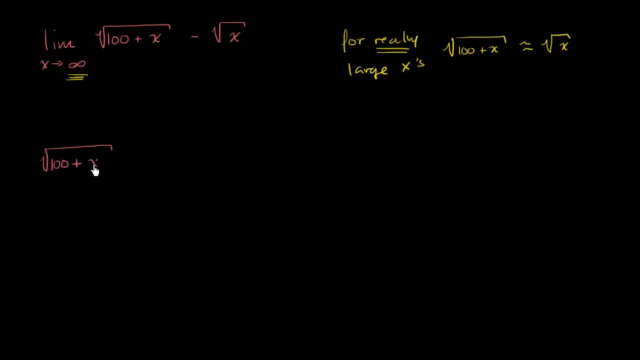 So this is 100 plus x, minus minus x. So one thing that might jump out at you whenever you see one radical minus another radical like this is: well, maybe we can multiply by its conjugate and somehow get rid of the radicals. 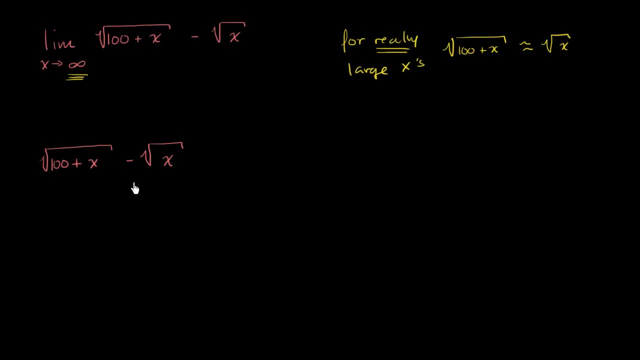 or at least transform the expression in some way. that might be a little bit more useful when we try to find the limit, as x approaches infinity. So let's just- and obviously we can't just multiply it by anything arbitrary In order to not change the value of this expression- we can only multiply it by 1.. 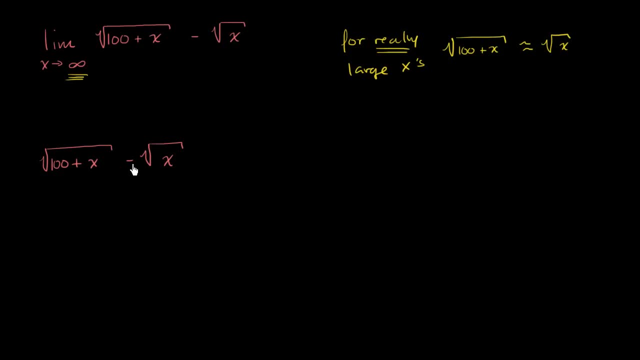 So let's multiply it by a form of 1, but a form of 1 that helps us, that is essentially made up of its conjugate. So let's multiply this. Let's multiply this times the square root of 100 plus x. 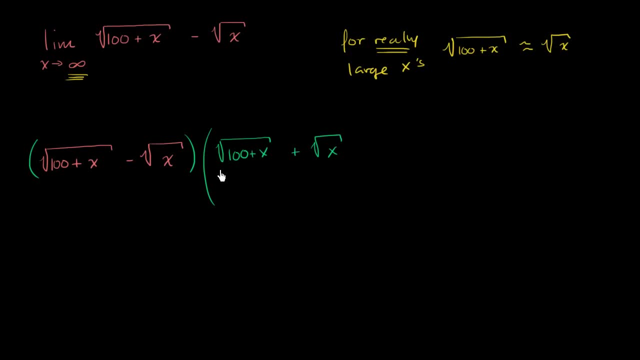 plus the square root of x. over the same thing: Square root of 100 plus x plus the square root of x- Now notice, this, of course, is exactly equal to 1.. And the reason why we like to multiply by conjugates is that we can take advantage of differences like this: 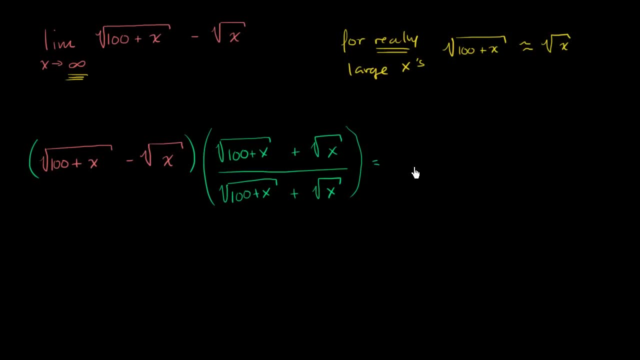 We can take advantage of squares. So this is going to be equal to: in our denominator, we're just going to have the square root of 100, let me write it this way: actually, 100 plus x plus the square root of x. 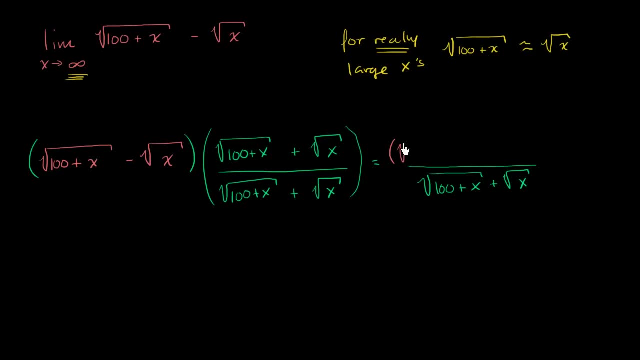 And in our numerator we have the square root of 100 plus x minus the square root of x. times this thing, times square root of 100 plus x plus the square root of x. Now, right over here, we're essentially multiplying a plus b. times a minus b will produce a difference of squares. 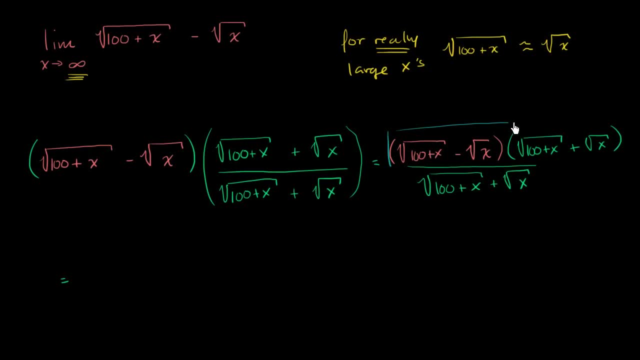 So this is going to be equal to this top part right over here is going to be equal to: is going to be equal to this. let me do this in a different color. it's going to be equal to this thing squared. 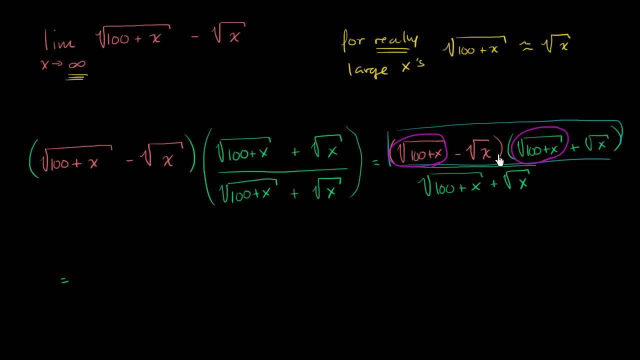 minus minus this thing minus that thing squared. So what's 100 plus x squared? Well, that's just 100 plus x, 100 plus x. And then what's square root of x squared? Well, that's just going to be x. 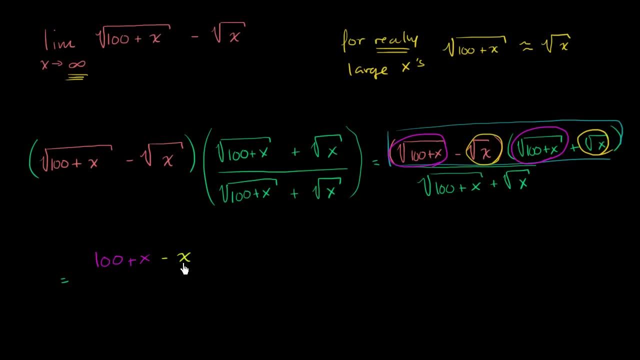 So minus x- And we do see that this is starting to simplify nicely All of that- over the square root of 100 plus x plus the square root of x And these x's, x minus x will just be nothing, And so we are left with 100 over the square root of 100 plus x. 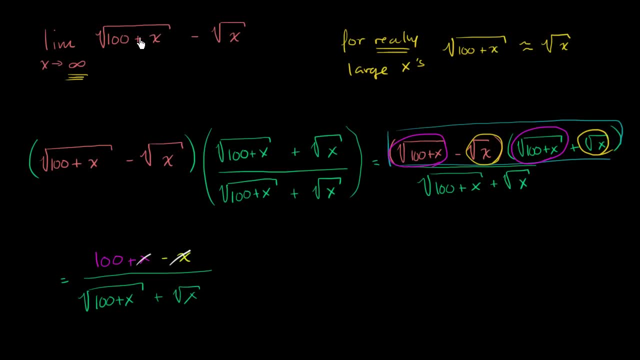 plus the square root of x. So we could rewrite the original limit as the limit, the limit as x approaches infinity. Instead of this, we've just algebraically manipulated it to be this: So the limit as x approaches infinity of 100 over the square root of 100 plus x.